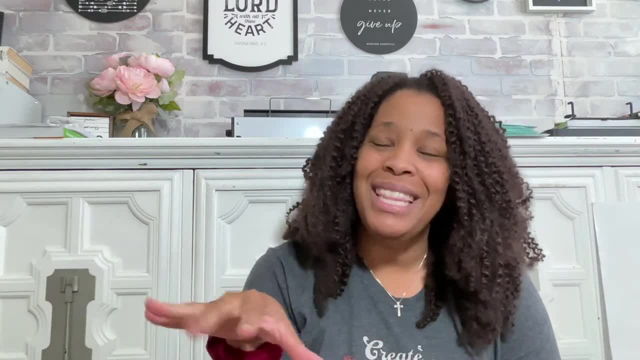 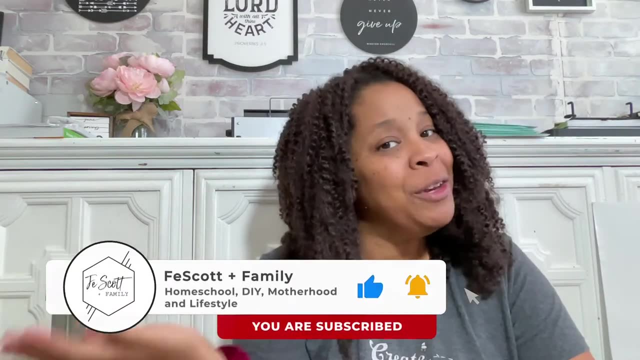 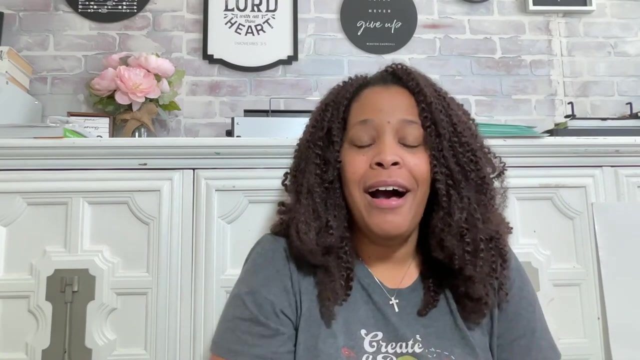 things, homeschool, motherhood and some fun DIYs sprinkled all up in there. so if you like that kind of content, then please like this video. subscribe to the channel. hit the notification bell so you don't miss out on new videos. so this has been a long time in the making. I mentioned in my update video that I'm 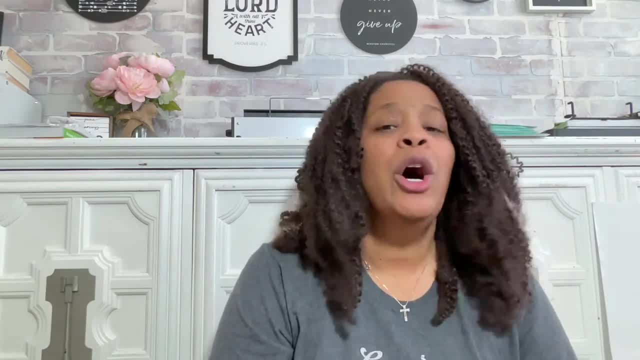 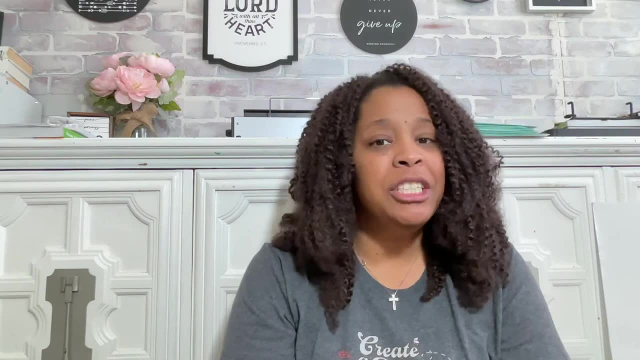 gonna start doing our own language arts curriculum that we're no longer going to use, a curriculum we were using to get in the beautiful, but we're no longer using that curriculum and you know, it has just been on my heart for a while to create my own curriculum. 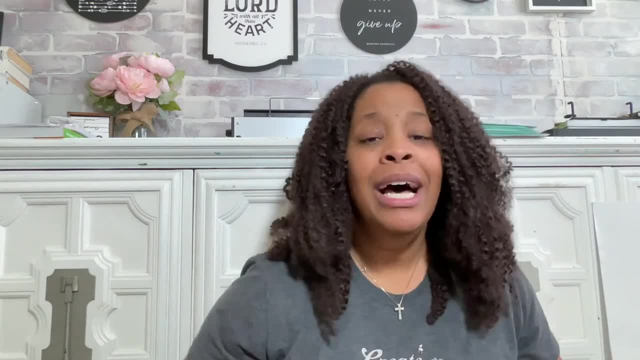 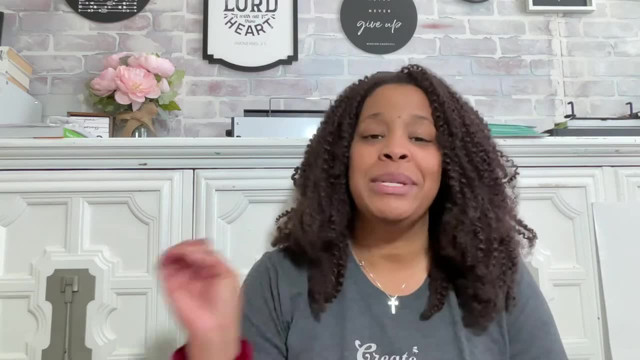 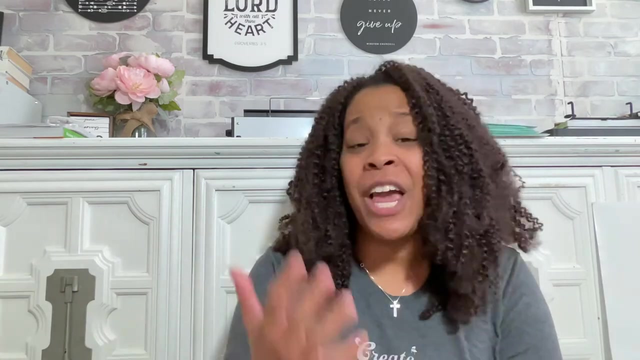 so, if you're still not part of my background, I'm obviously going to share a few really interesting lessons now based on that, because I want you to do the same thing for history and I'm slowly kind of working my way through that as well. we're using sunlight as our base, but I'm building onto that. 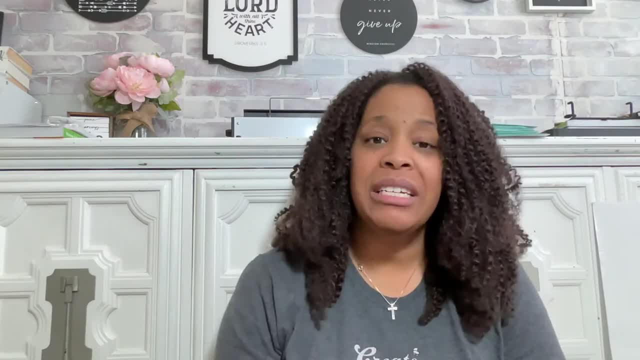 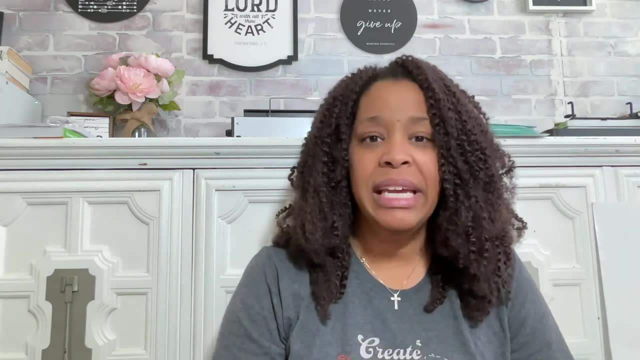 but language arts we are 100 percent doing our very own curriculum, so no open and go. I am putting things together for that and I thought I would share with you the resources that I'm using to create our very own language arts curriculum. I'm actually going to do this video, probably in three È'n. 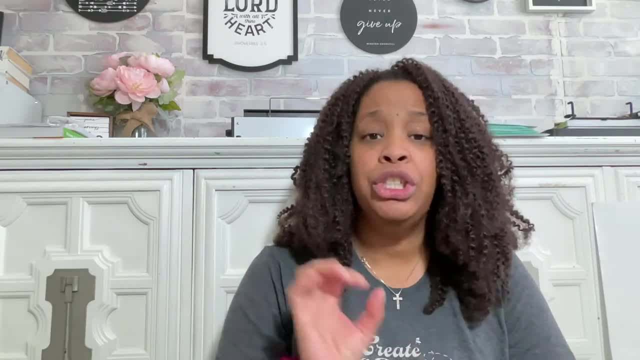 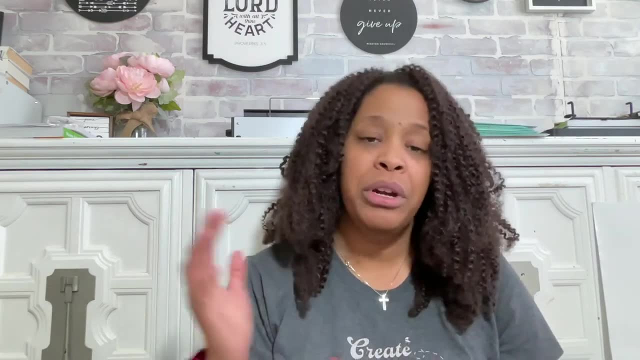 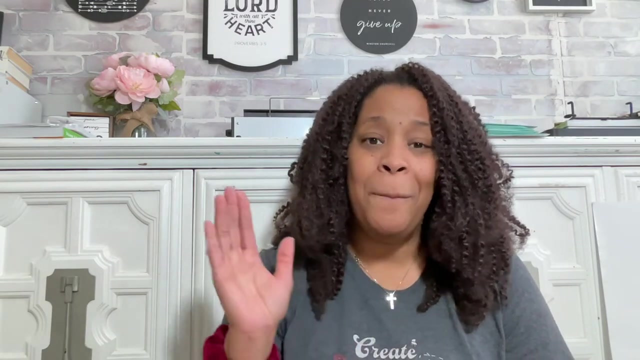 three parts. i'm going to do this one here, which is showing you what i'm using to build our curriculum, the resources that i'm using, what i'm using to make sure that we're staying on track, that we're covering what we need to cover, all right. and then i'll do um two videos that will be broken down by: 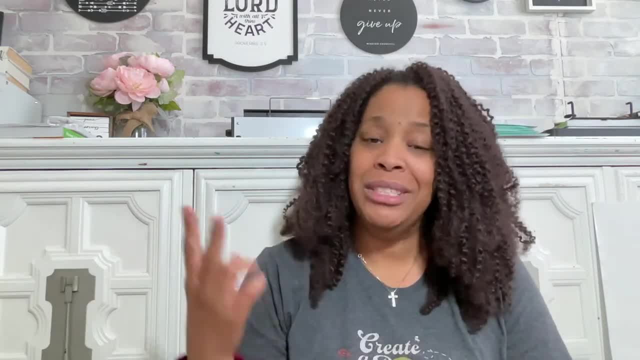 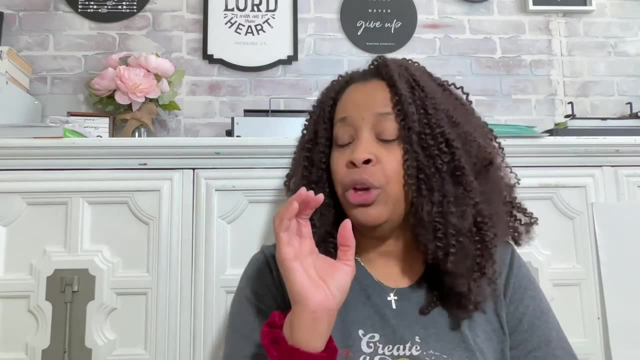 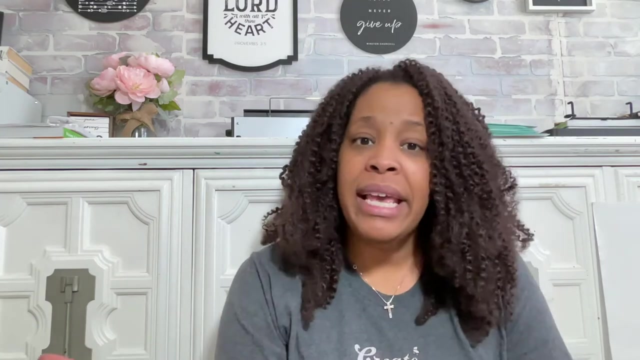 grade level. so it'll be for kindergarten and for third grade, which those are the grades i have for kids right now and i'll show you specifically what i'm using for each grade level, um showing you the uh like where i'm getting worksheets from, um any type of writing things that we're using. 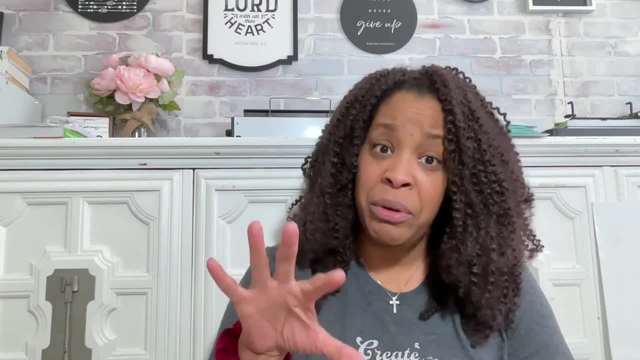 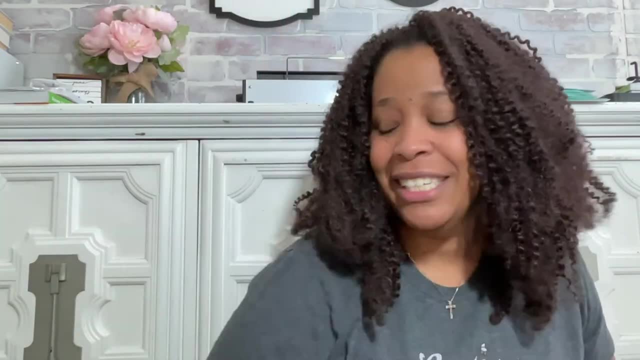 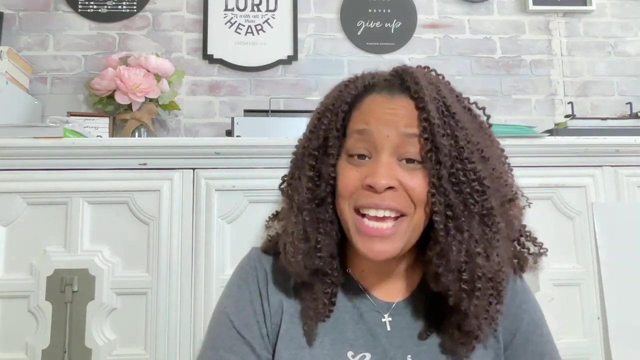 anything that's specific for that grade. i'm going to kind of do separate videos for just kindergarten curriculum and third grade curriculum. so sorry, i talk with my hands a lot. um, anyway, guys, i am excited about this. it is- it is time consuming, it has taken some time, but i'm really happy with. 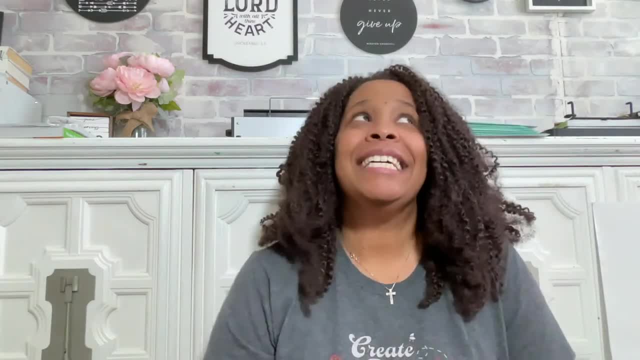 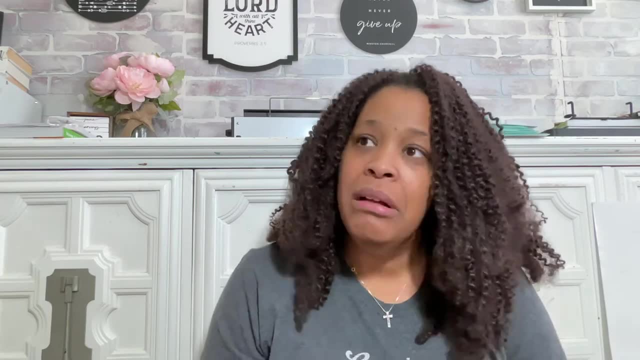 the progress that i've made. i'm really happy that i have like, uh, you know, just went ahead and did it, because i have been like so scared and i'm still scared. i'm like, oh my gosh, like what if they don't learn anything? i don't, and you know what. and if 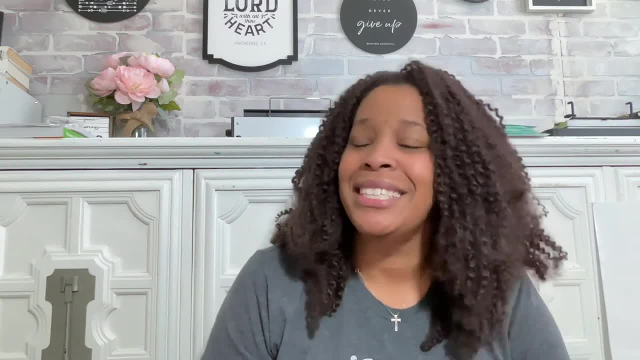 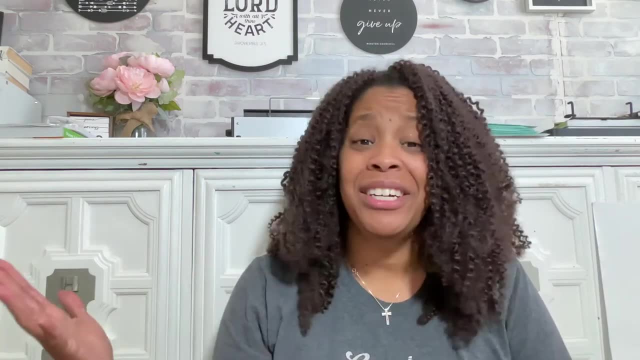 they don't learn a lot this year, it's okay, because you know education's all around us and they're they're going to learn something one way or another. they'll pick up something this year, whether or not it's everything that's on our checklist or if it's just, um, you know a couple. 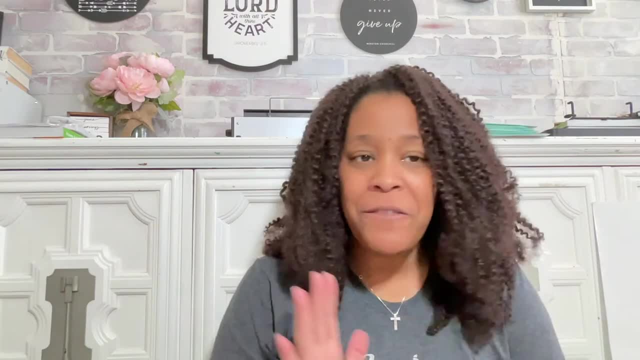 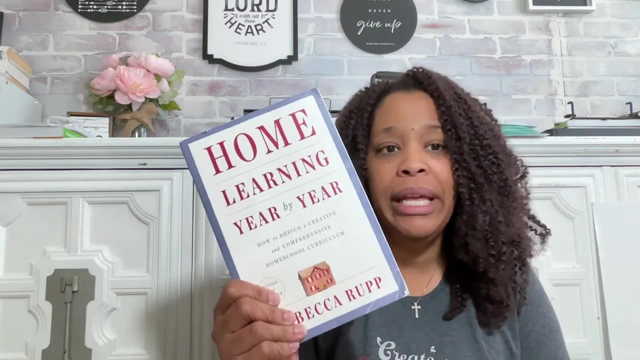 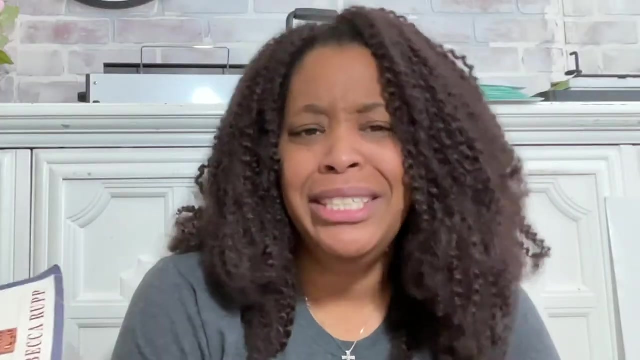 things, but they'll be okay. kids are resilient, all right. so the first thing i'm going to show you is- this is the first book, and i have showed this up on my instagram before. this is home learning year by year: um by rebecca rup rup. it's great for your teaching language arts and you can't even read. 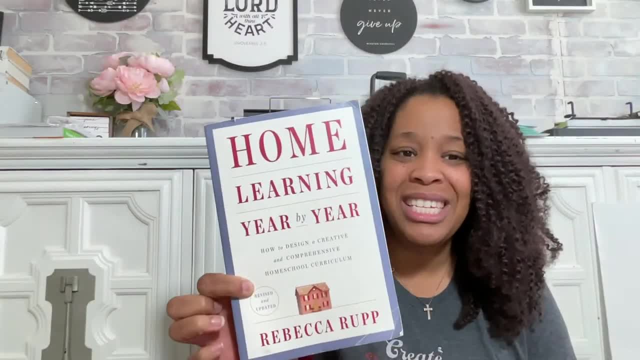 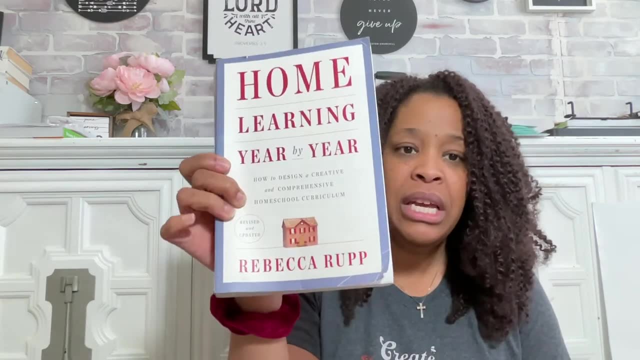 um, okay, but this is the book that we are using. this is the revised cop, revised and updated one, so this one was 2020, so the first one's from 2020 and then from 2000, and this was 2020. it's updated. 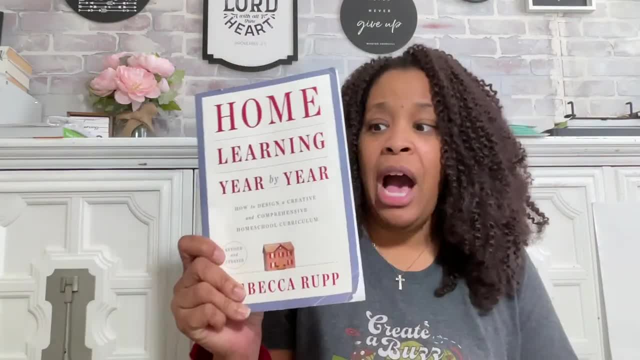 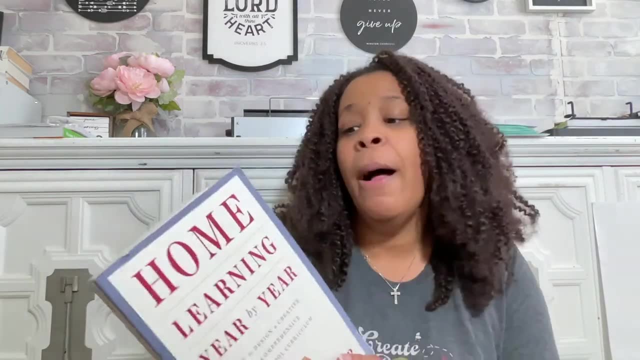 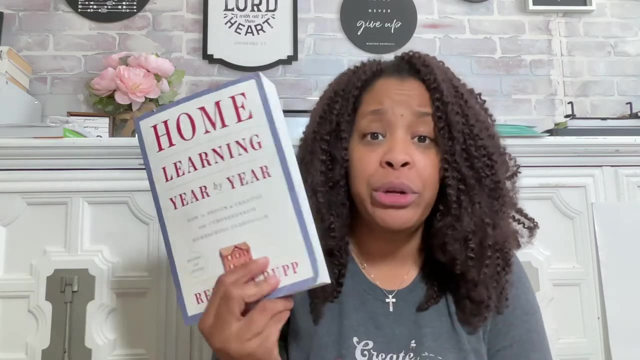 i've mentioned in the past, especially following on instagram, how i like to look at this as a guideline. it is not the holy grail, it's not your end-all bible, but it is a very great space to start when it comes to building your homeschool curriculum for your child, and this covers every. 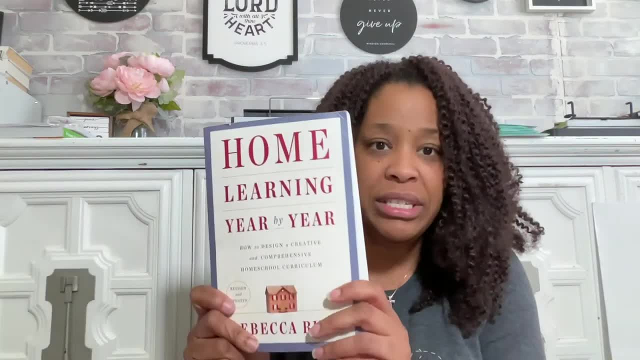 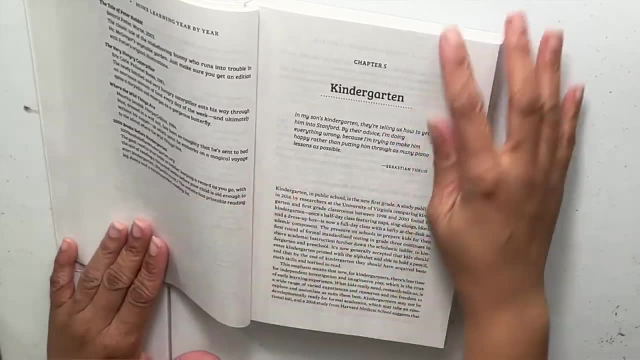 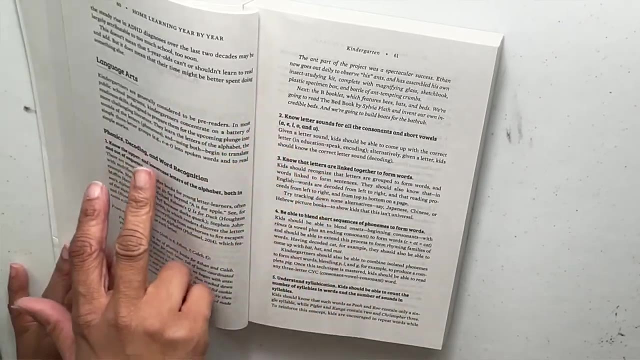 um subject, so not just language art. so this covers every subject for your child and it will let you know um when you go say, here, here's kindergarten and then, um, it kind of breaks it down as to what they should be learning as far as, like, language arts, phonics, decoding, word recognition. so they should know the upper and 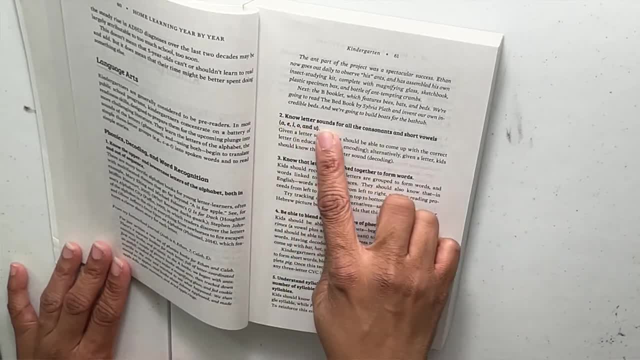 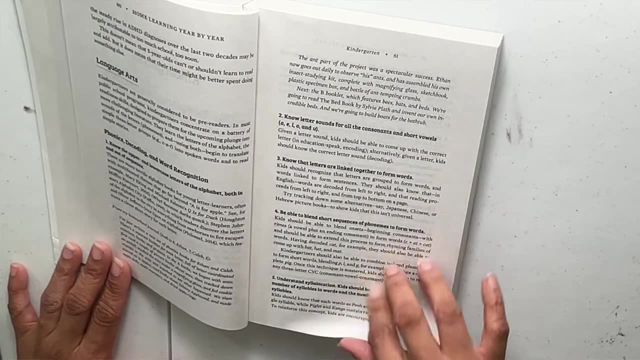 lowercase letters of the alphabet, both in and out of sequence sequence. know the sounds of all consonants and short vowels. um, know that letters are linked together to form words and it kind of just gives you a breakdown of things and also will have a list of resources, um, back there that you. 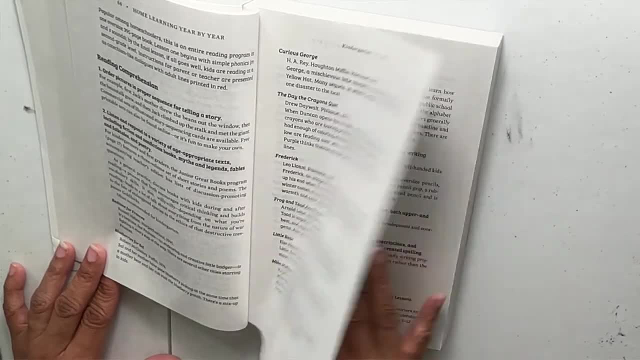 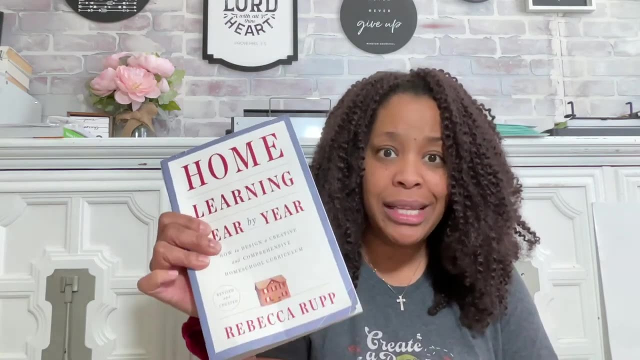 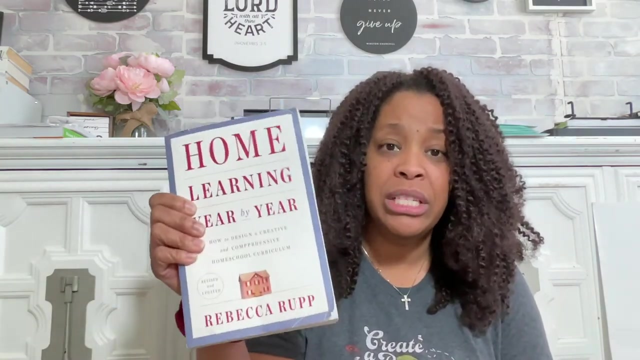 can also use to help with building your curriculum or teaching. and then when you go say here's kindergarten, and then it kind of breaks it down as to what you're teaching, said subjects, uh, um, and i really enjoy this because it does give a really great checklist- and what i did is i went ahead and just kind of created a checklist for these subjects or 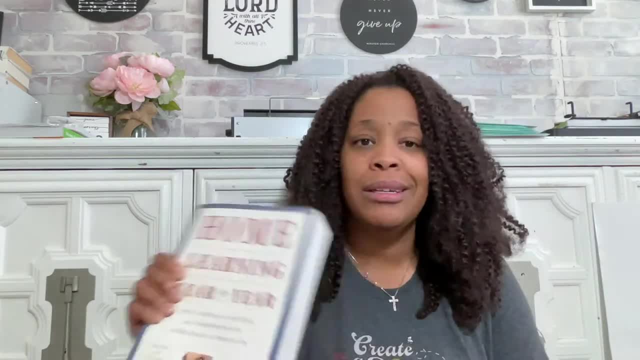 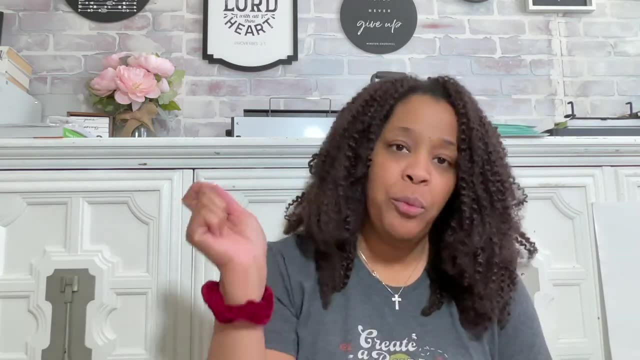 for this grade. so i had language arts and i just kind of wrote out on a little table, um, what skill they should should be learning, and um left a box: whether or not we've already mastered that, we're kind of like intermediate with that or we have like completely mastered that, and then i just kind 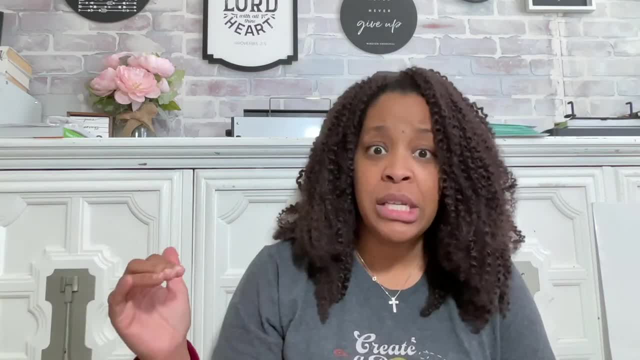 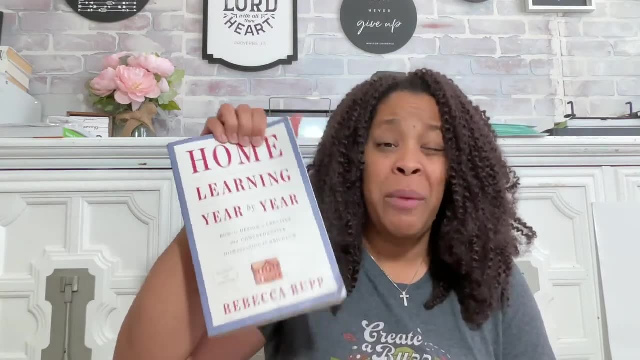 of went ahead and just kind of wrote out on a little table um left a box. whether or not we've already mastered this, you know this subject or this um, this skill set and we can move on to something else, or we need to do more work on it. but i'm just using this as a great guide to make sure i'm 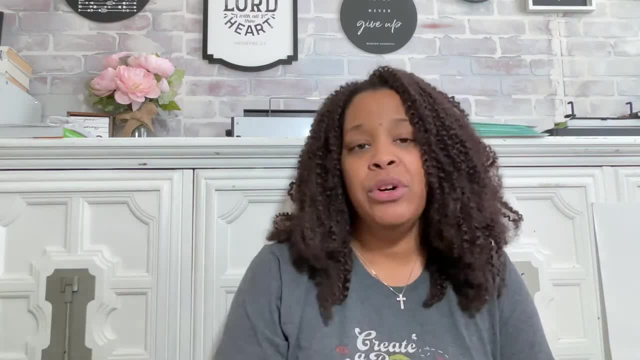 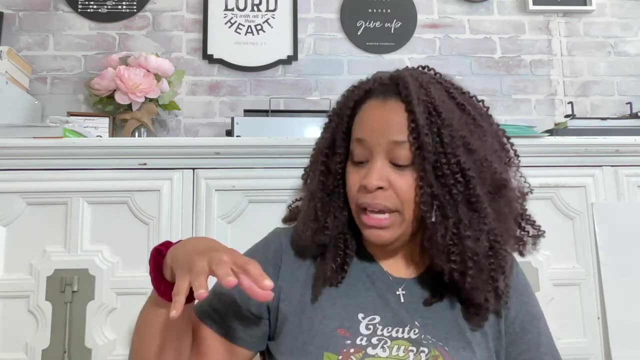 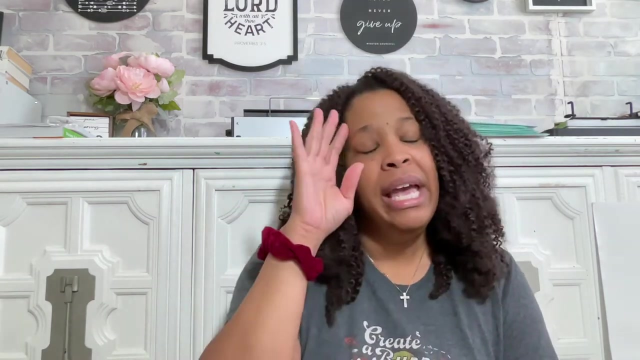 covering a lot of what should be covered at grade level. and again it's: there's always going to be gaps in education, there's always going to be gaps in learning. but, um, i'm using this again, not as the be all holy grail, but as a great guide to say, okay, this is kind of giving me a roadmap of what i'm. 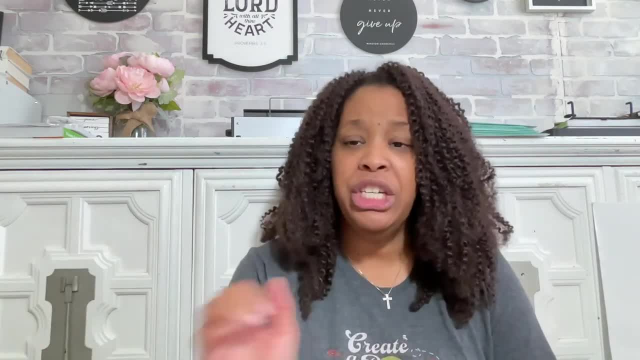 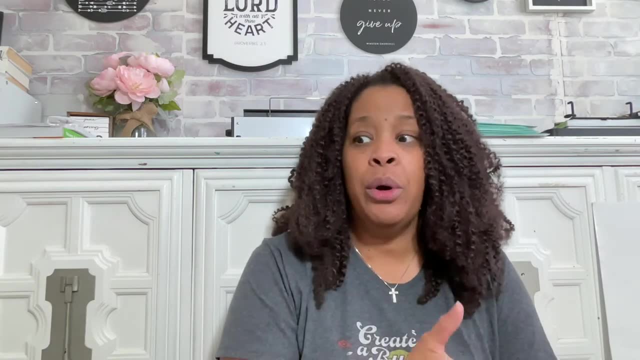 going to cover whether or not we cover all this this year, or we just, you know, sprinkle a little bit of this in, or some things your kids already know, even though, okay, they say it's for a third grade level. maybe they learned that in first grade or second grade and they're like they've mastered. 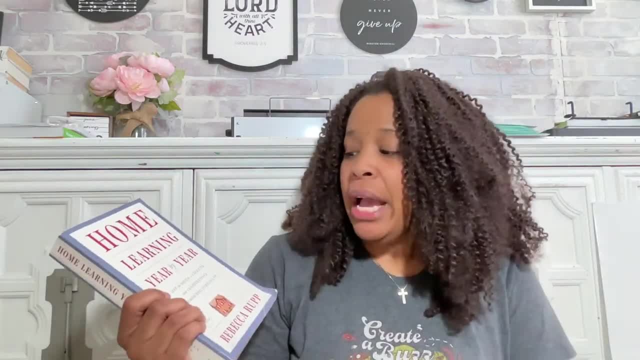 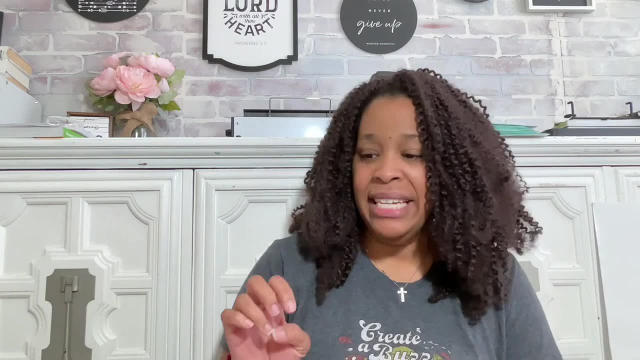 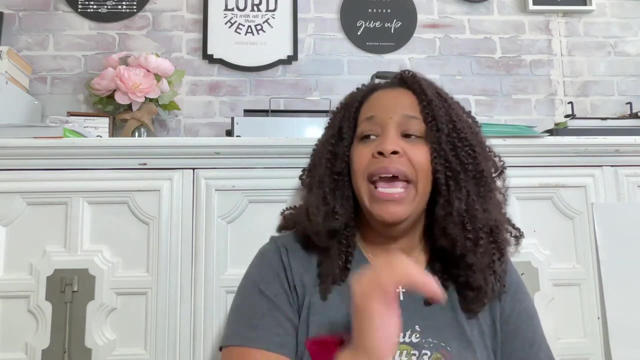 that a lot of this in here too. it's kind of giving you a guide to what it's saying, like what they should know by this grade. i don't think that it's they absolutely have to learn it in third grade, have to learn it in kindergarten or have to know it in first grade. it's like, hey, usually around this. 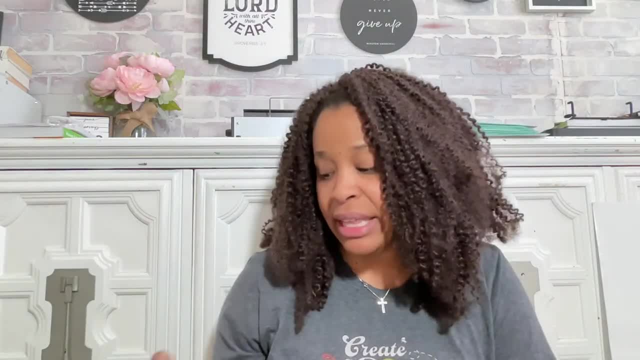 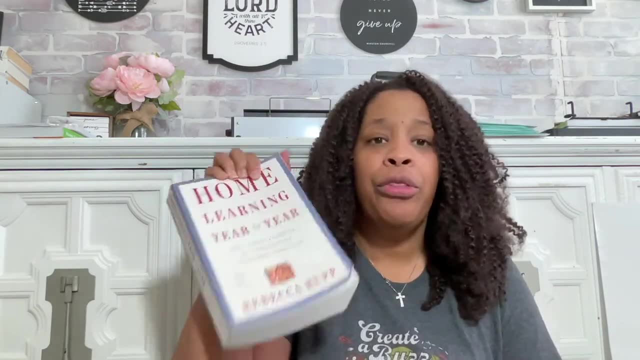 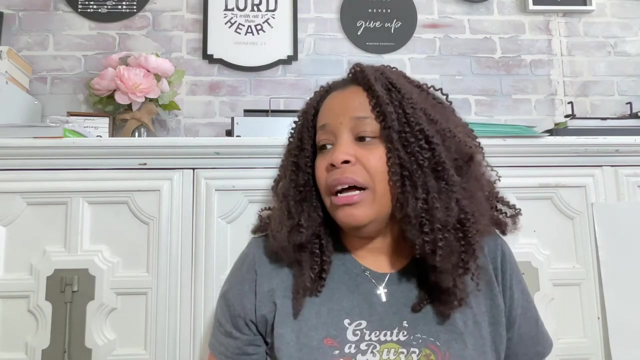 time. this is when kids are learning this. so, again, i think that this is a great roadmap. um, it's not the end, all be all. so if your child is in you know third grade and they have not mastered multiplication, or they have not mastered um, uh, you know punctuation or whatever, like, don't feel. 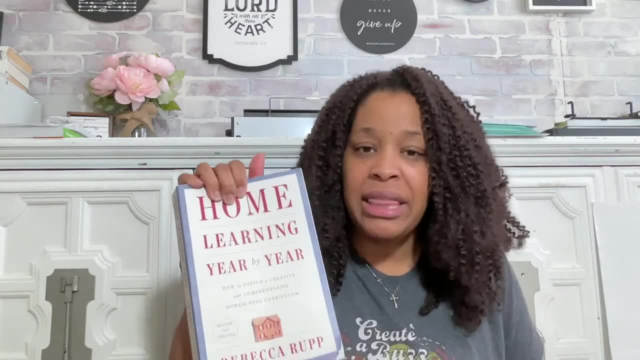 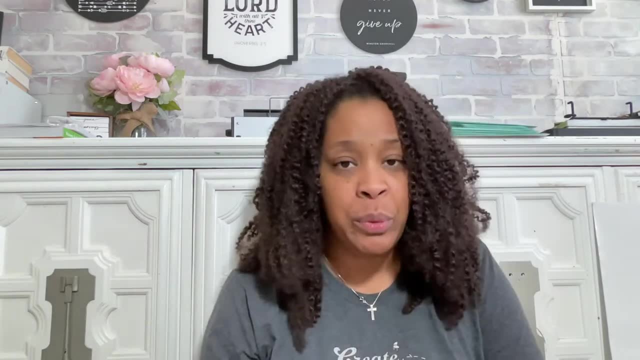 like, oh, they're behind, just use it as a guide, like, okay, that's something that i want to make sure i cover, and then i keep covering, covering, until they get it. so if they didn't get in third grade, we're going to move it over to when we do it. 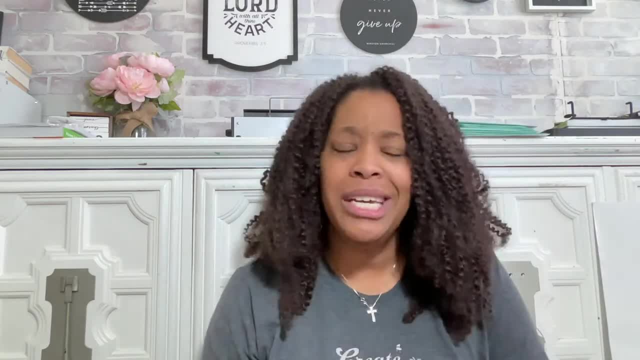 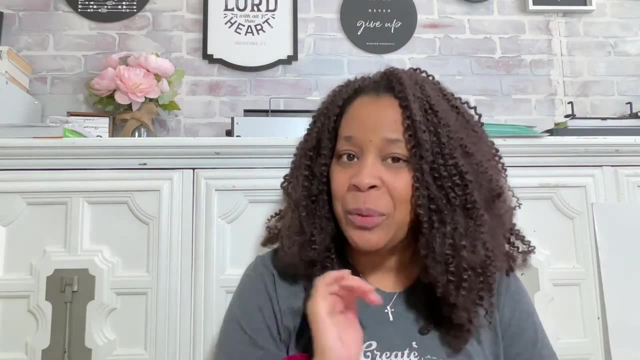 next year for fourth grade. if they didn't get, you know, all these sight words in kindergarten, okay, we're going to move those over and put those in first grade. so it is a roadmap, but it's not the be all end all, be all, all right. next, books that we are using for resources are the um. 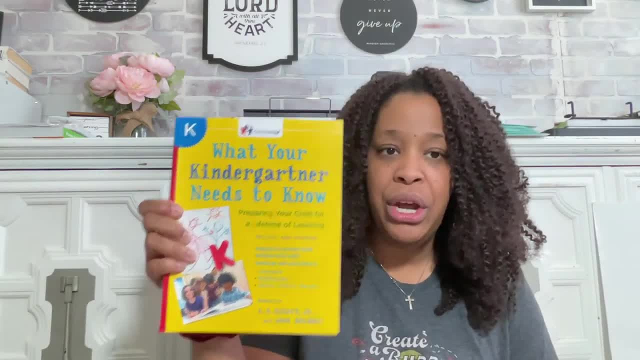 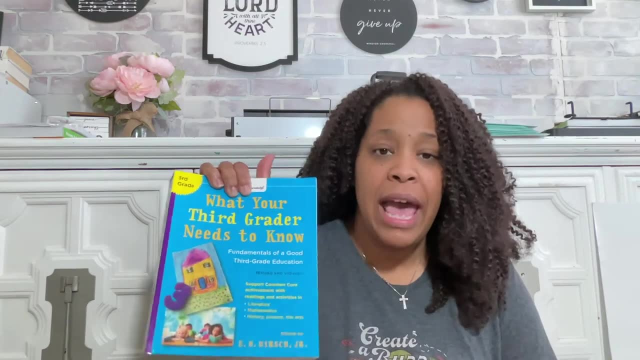 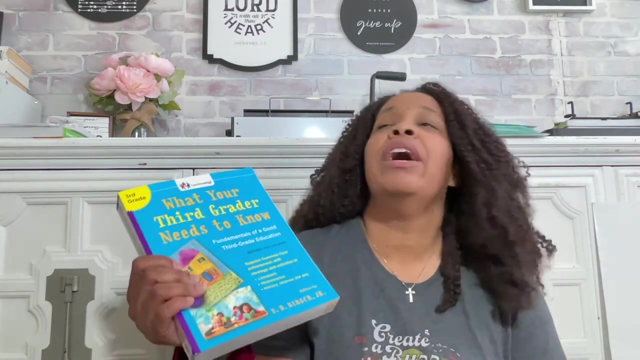 what your kindergartner needs to know, and then we have what your third grader needs to know, so they they have these books in every grade level, from kindergarten to sixth grade. what i like about this is not only does it kind of say, like okay, for third grade language arts, these are the things that you should cover, it also gives examples, or 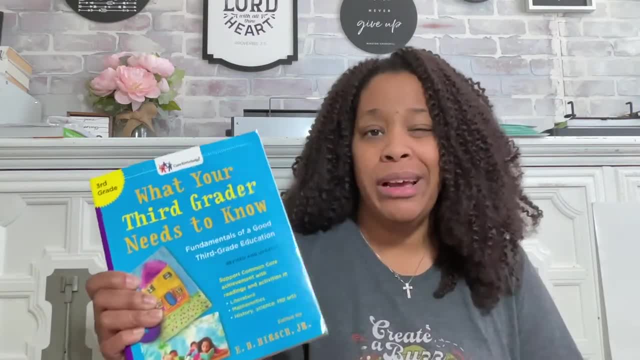 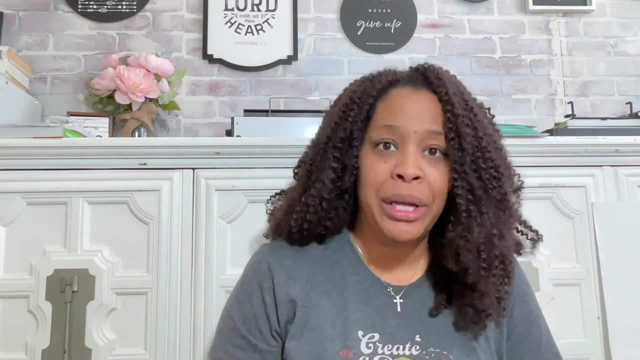 actually almost kind of like mini lessons in here, so this is almost like a lesson book in a sense that you can take from it. um, so say, for example, we're actually learning about the pilgrims right now, and i'm going to be learning about the pilgrims right now and i'm going to be learning about the. 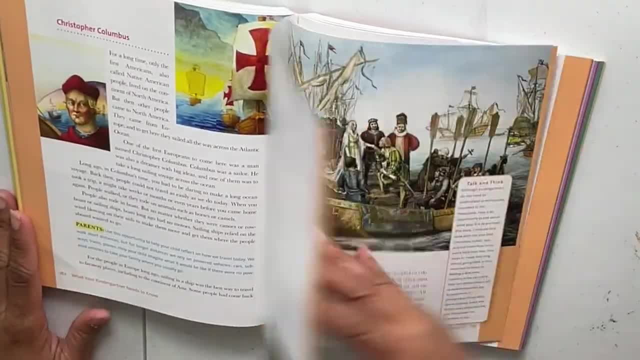 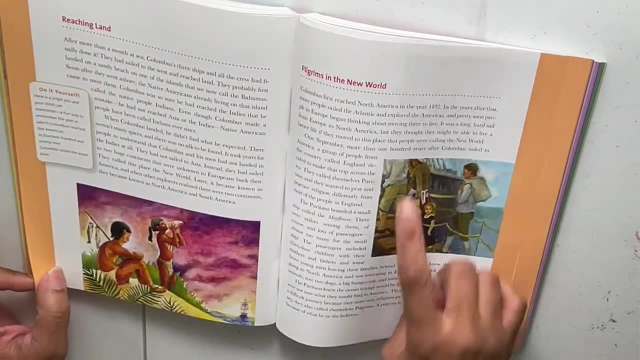 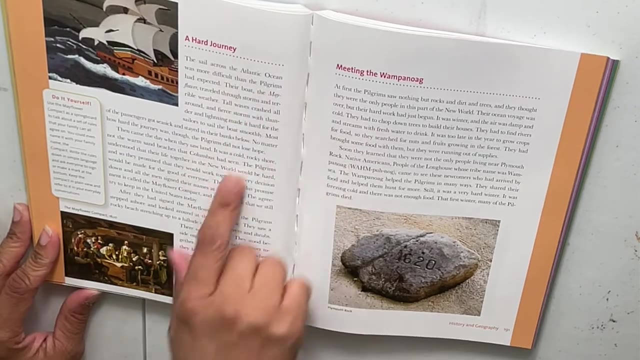 pilgrims right now, and i can go into the kindergarten book right here and um learn about the pilgrims. there is a spot about pilgrims in the new world and here is a part that i can read. i can read about this here and then on the next page it shows: you know, do it yourself, use the mayflower. 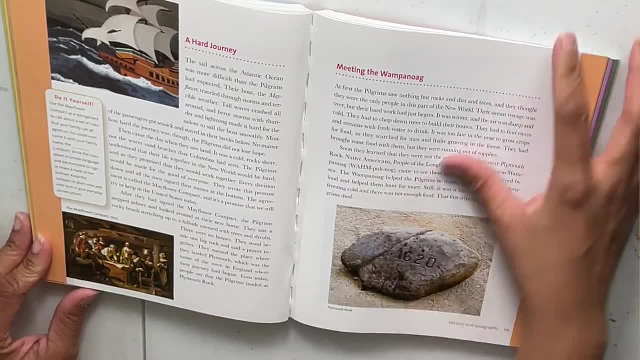 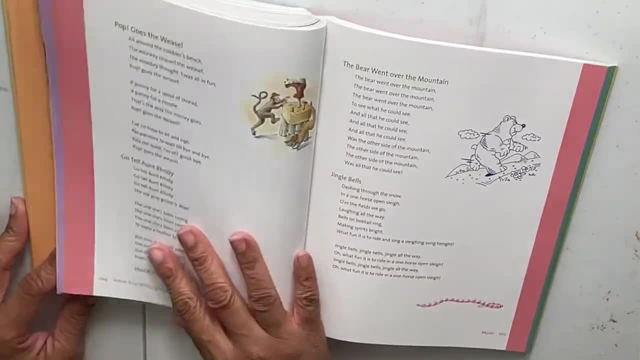 compact as a springboard to talk to your kids about setting rules you know for your family. so it has excerpts of poems, short stories all the way through, and then on the next page it shows the classics. in here, um, it gives examples of things to um, assignments that you can do, and 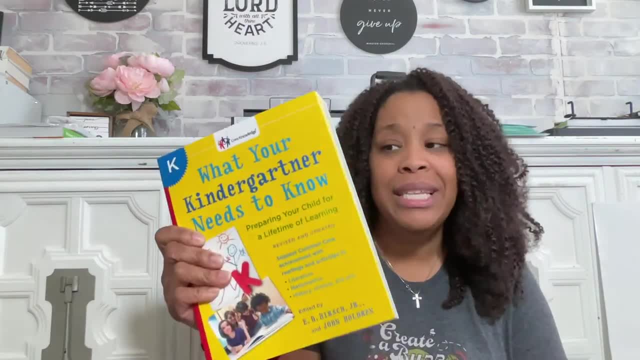 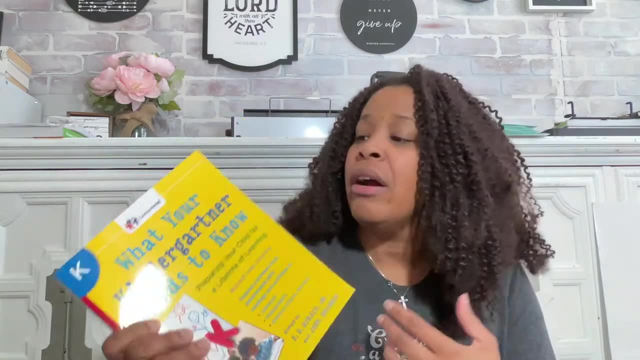 lessons that you can make. so you could almost use this as um. if you wanted to use this fully and solely as your curriculum, you could. it has great examples in here. it kind of walks you through um it is, you know. it says it supports common core achievement with reading and activities. 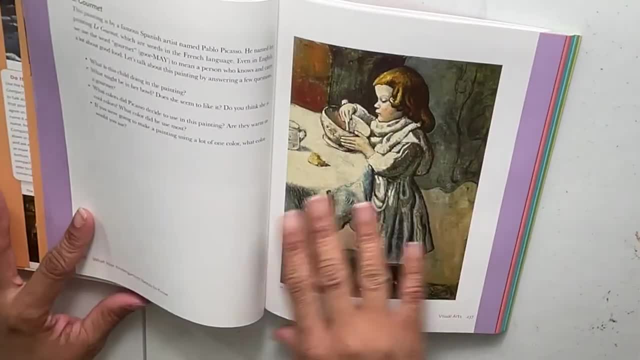 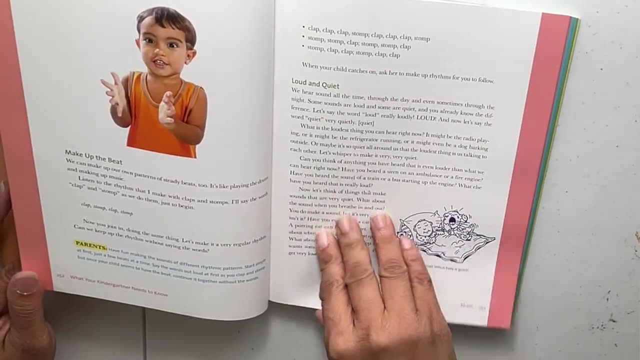 and literature, math, history, science and the arts. it even has, like, visual arts and music, so it has nursery rhymes and those songs and things to help you with with building a music curriculum or teaching music and visual arts to your kids. um, so these are great because they do they cover. 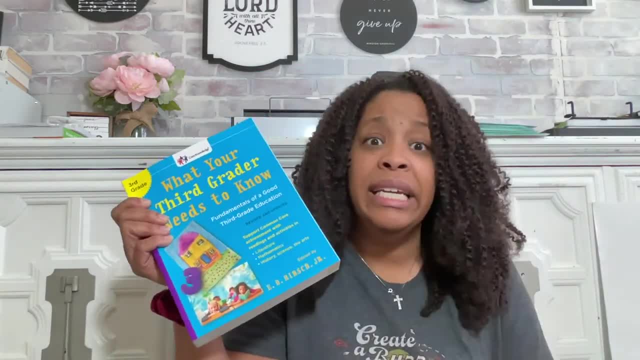 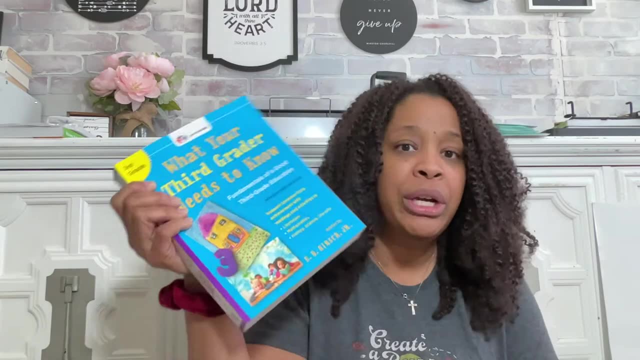 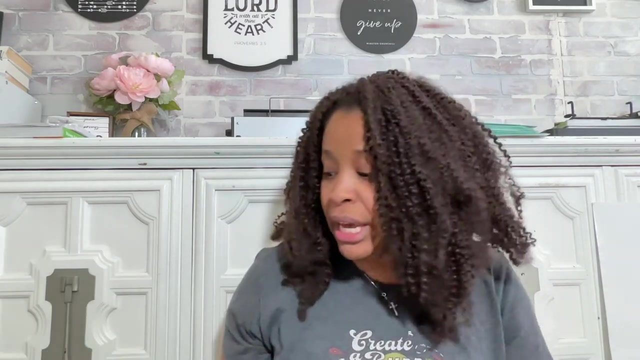 they kind of show you what you uh need, what, what you should be kind of covering at this grade level, and it also gives examples and excerpts of like literature and classics and things to read, as well as kind of like lessons and little hints of what, how you can um teach those things to your kids. 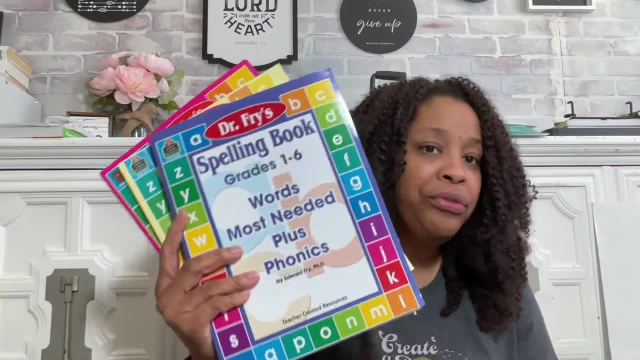 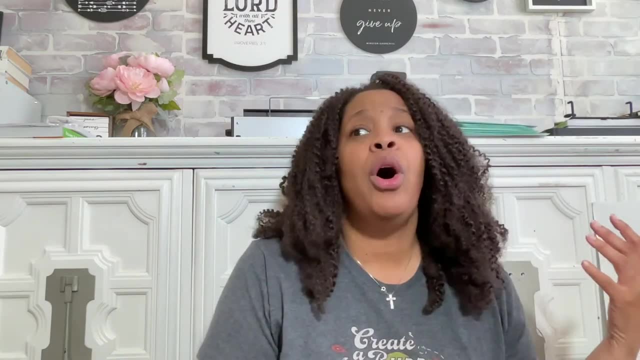 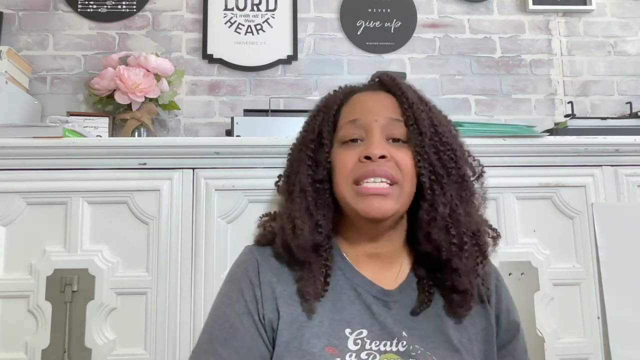 also using a few of the dr fry books and i'll show you these individually just a second. but the reason why we are using dr fry um over dolch sight words or reading is because i have chosen to use fry sight word because fry sight words are um most recently updated. there's a bigger list of words taught at a. 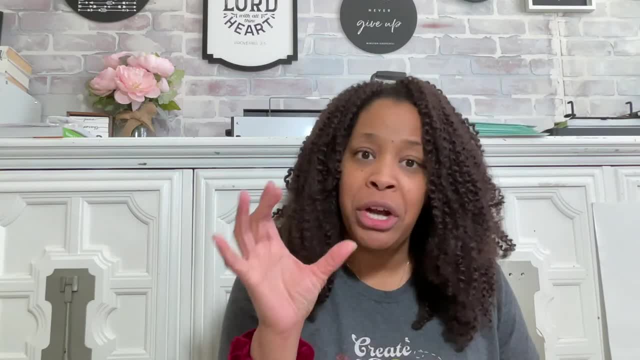 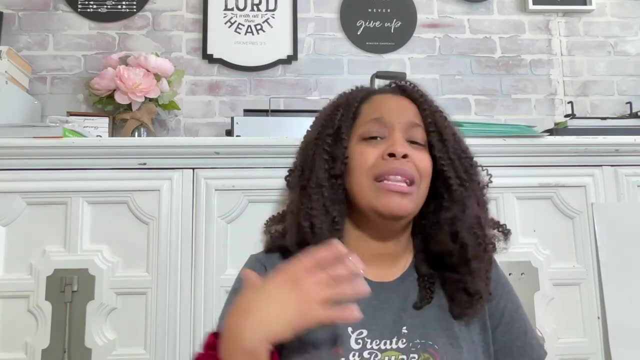 smaller, um, you know, in a smaller section or a chunk, so like five words at a time. and um, they're just some of the most frequent words. so we have just made the decision to use fry. a lot of people still use dolch, but dolch, but it's kind of up to you. 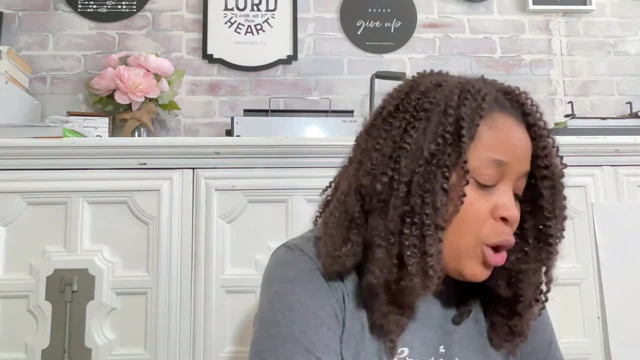 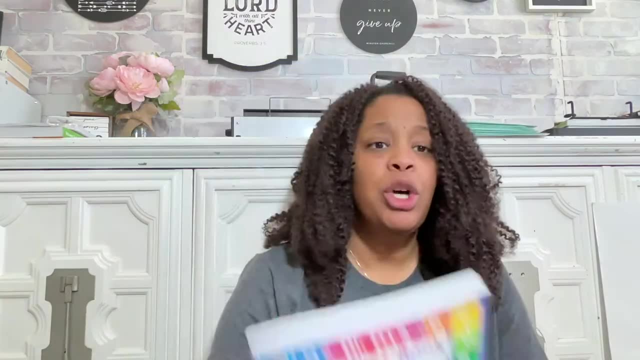 as a person to prep. it's what you decide to use, but we're going with fry words, so we are using fries. um spelling book grades one through six words most needed, plus phonics. so what's great about this is you will actually. it has a test in here so you can actually test your child to see. 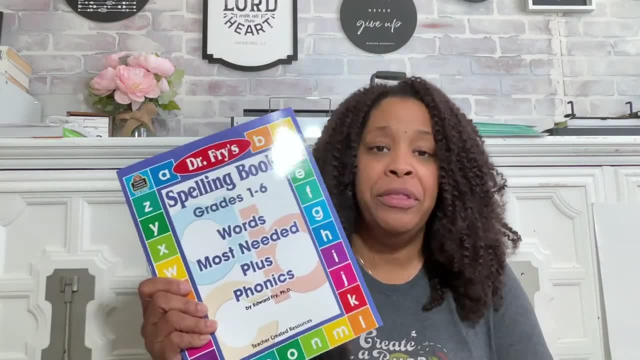 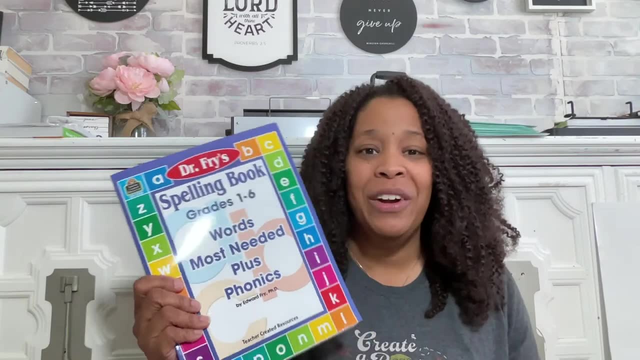 where they fall, what words they know, you'll know whether, to put them, you know level one, level three, because the the levels don't necessarily correlate with the grades. so just because you know they're in grade three, it does not mean that they're going to be on level. 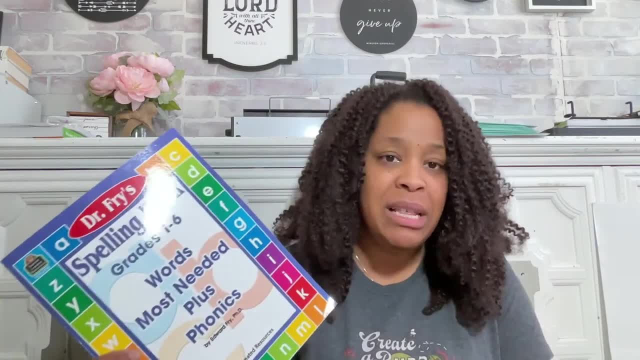 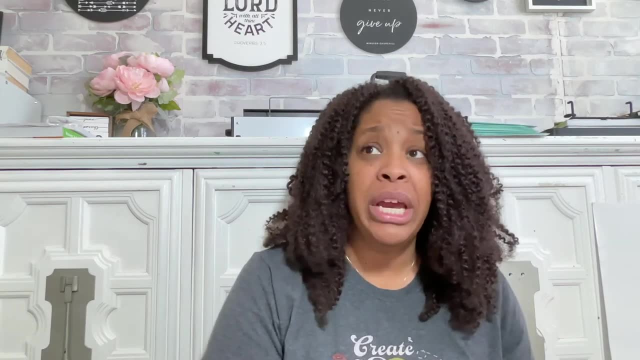 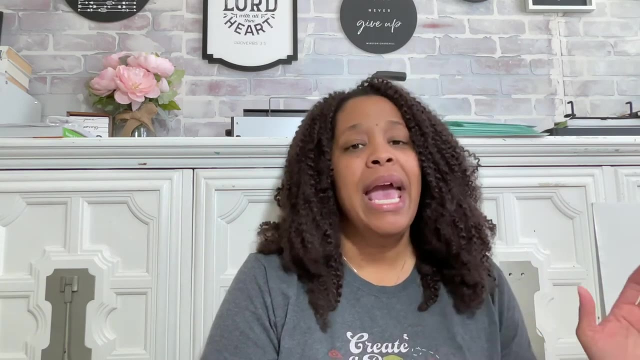 three spelling words, um, you know. so there's a test in the back. you can kind of test and find out where they fall. so for kennedy, when i tested her she actually got all the level three correct and, um, she missed three, i think, of the level four. and the way it is is basically, if you miss three, you 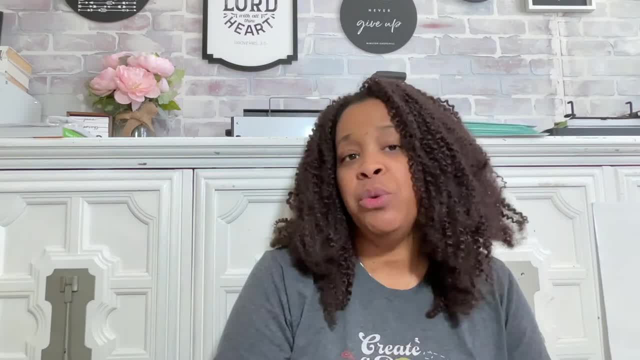 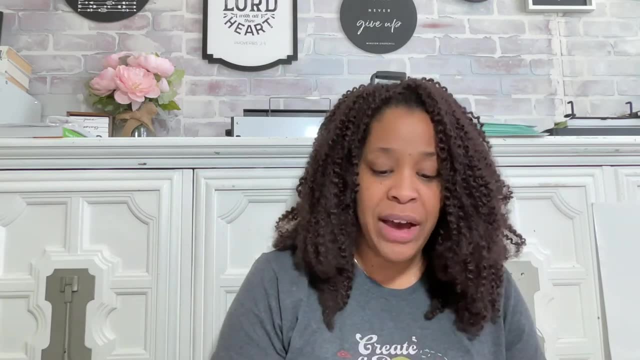 can start at that level, but she made the decision that she wanted to actually start at level three. so for her, what we're doing when we're using this spelling book, i i'm just going through level three. i'm finding the words. it's uh, 20 words and i'm just going to that 20 and whatever words she does. 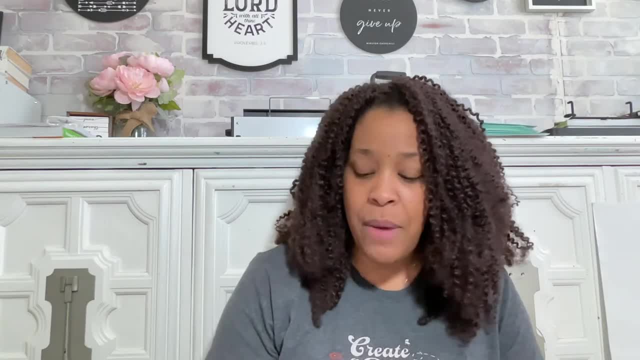 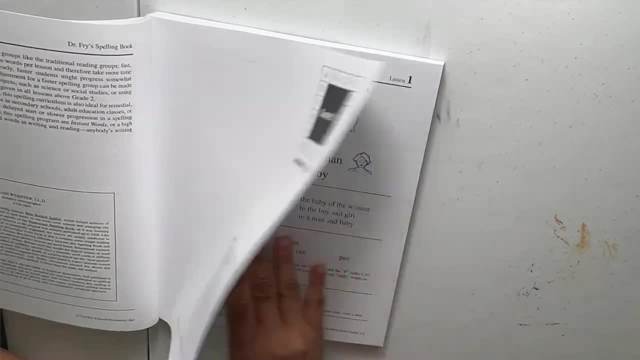 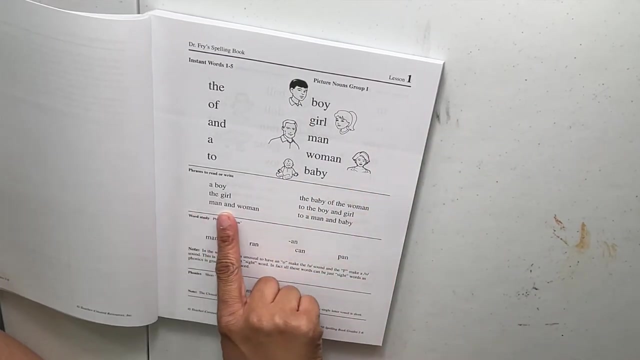 not know out of that 20. those would be her spelling words for that time. so, um, the way it's broken down is: you can see here, so this is level one and you have, um, instant words or sight words over here, noun words, and then it kind of tells you here: um, you can see here what level three is. 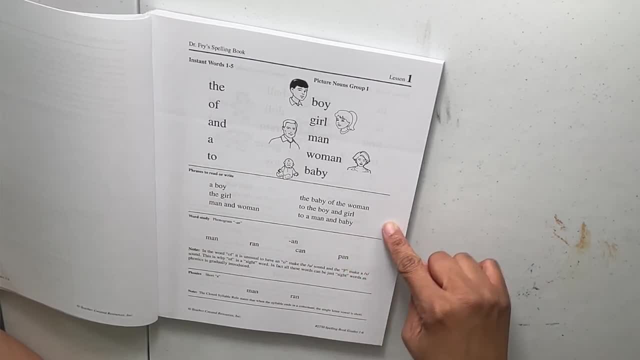 please uh phrases to read or write that they can practice. you know, here it works on phonograph phonograms, so there's always a word study section right here in the middle and then there's phonics at the bottom, so depending on what grade level. so this one has. 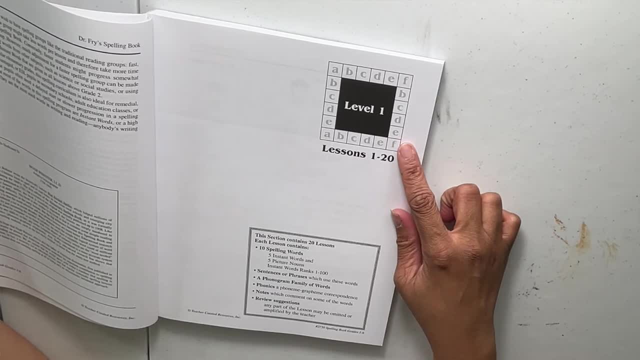 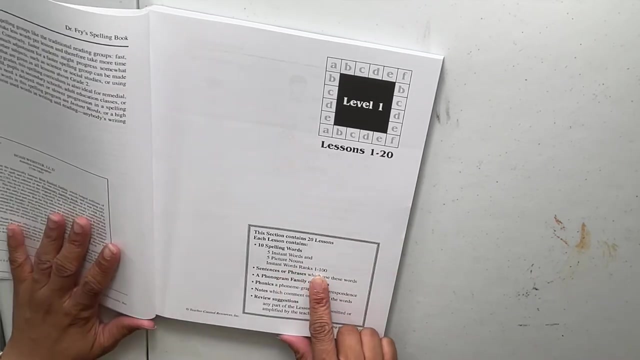 on the first page. here, level one, it kind of tells you what this section contains. this section contains 20 lessons. each lesson contains 10 spelling words, which are five instant words and five picture nouns. instant word ranks um one through 100. so these, so this level will cover all. 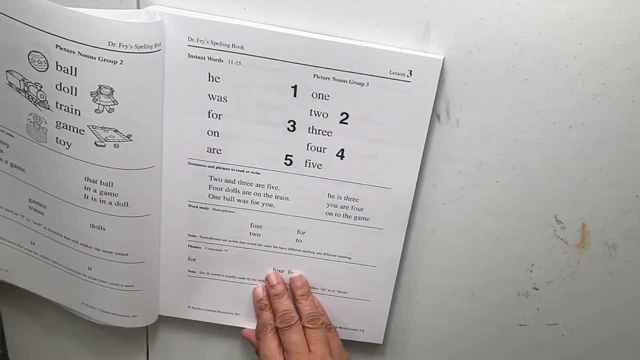 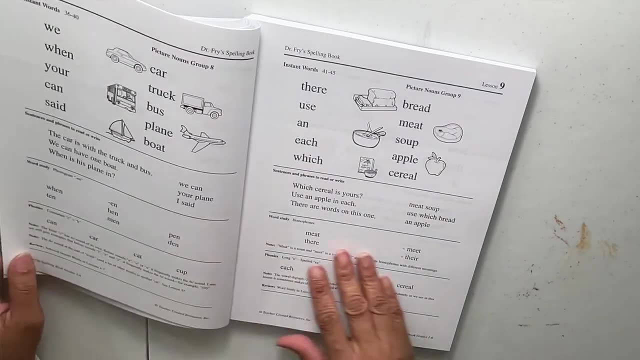 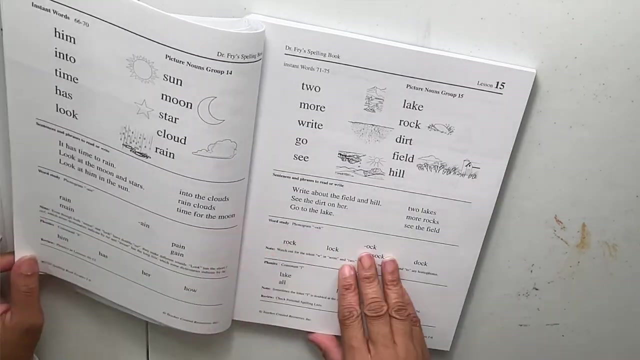 of the first 100 of fry's spelling um, instant words or sight words. it has sentence or phrases which use these words, a phonogram, family of words, phonics um, notes and review suggestions. so it kind of covers everything right there, tells you what's in there and then, if you skip up, 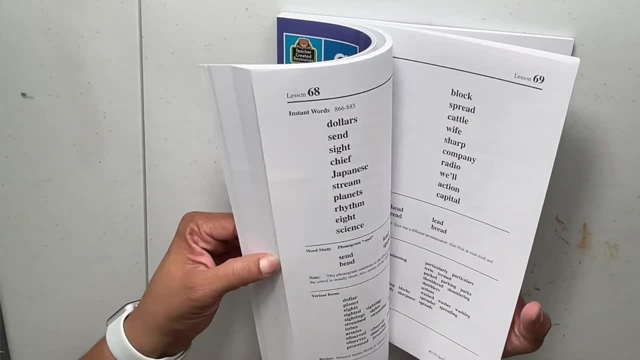 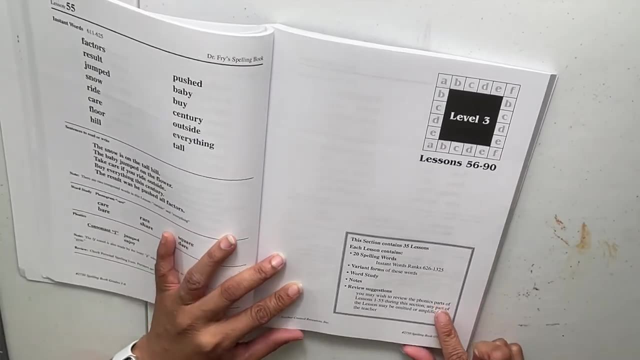 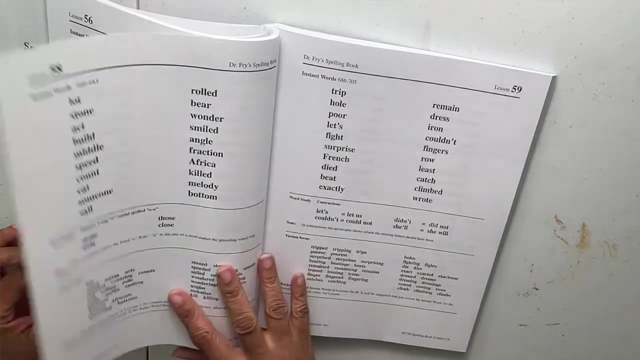 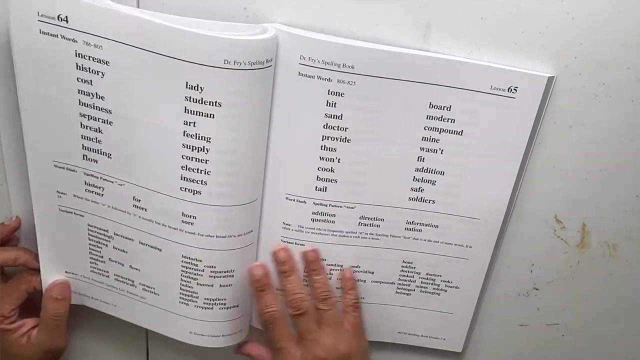 we'll skip up to level three. just kind of give you a show of what that looks like and what's in there. uh, we have level three. level three uses, uh, 20 spelling words. it's the instant words rank from 626 to 1325. there's a variant forms of these words- the word study, so it'll talk about. 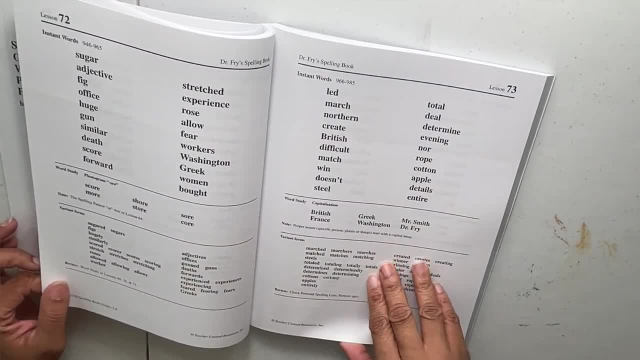 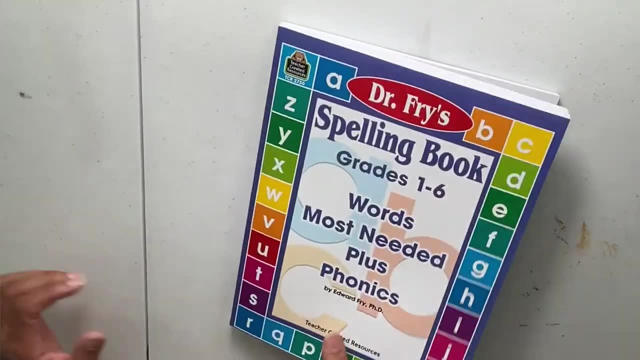 synonyms or antonyms or homophones, like different things for the word study. you can do like you know, just kind of give you some review suggestions down there. so these that's how this book is broken down. so we are using this for our spelling words to make sure that the girls 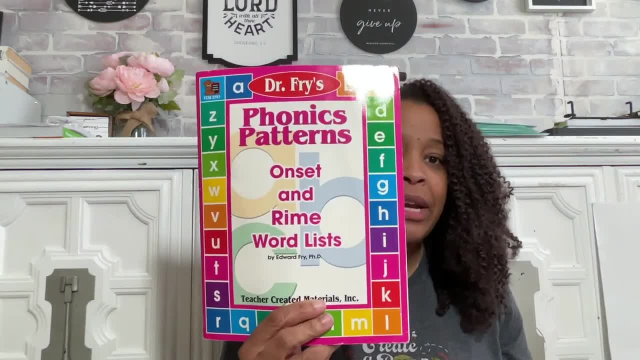 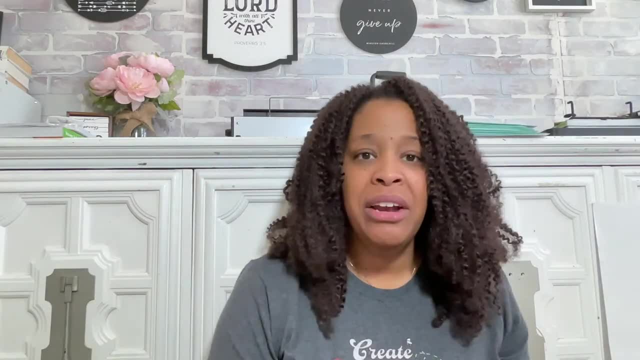 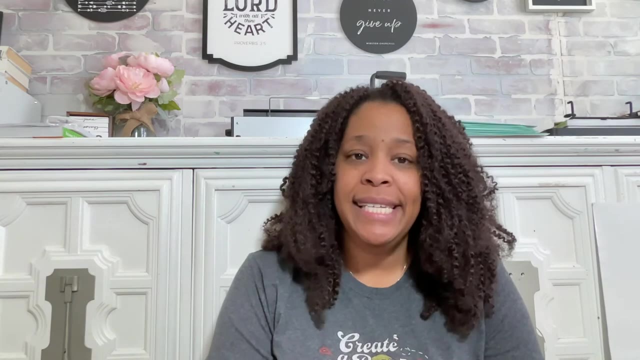 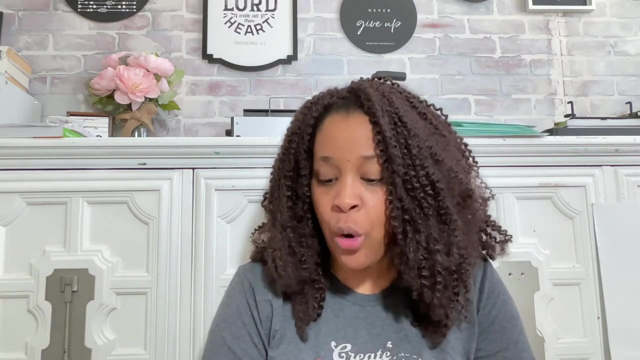 can spell this book here: phonics patterns, onset and rhyme word list. and again, this is um. basically the idea behind phonics in you know word families is: you know, if your child can read a- t and they know c a t is cat, then they'll know m a t is mad and h a t is hat and that kind of thing. so this: 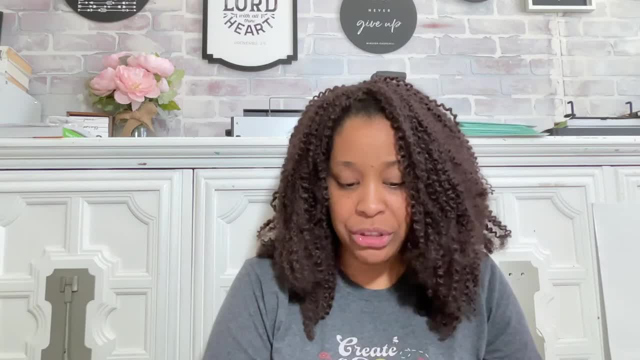 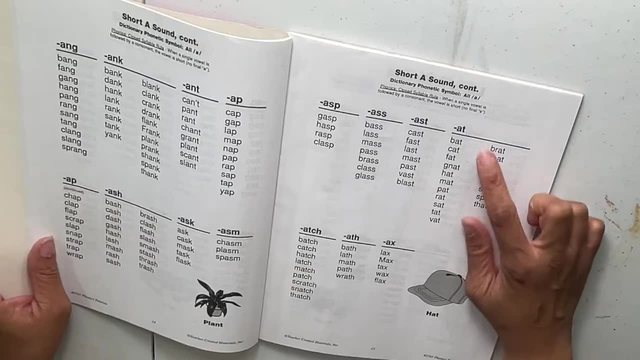 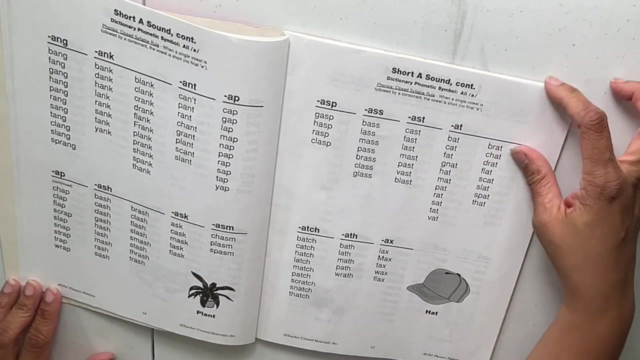 gives you, um, just a great list of word, families basically, and that way you can you know. so here we go, you have hat, or you have, you have at, you know at family over here, and then you know you. this way you're able to, um, you know, kind of. 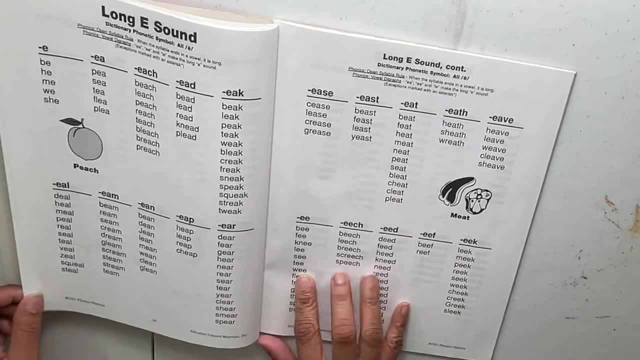 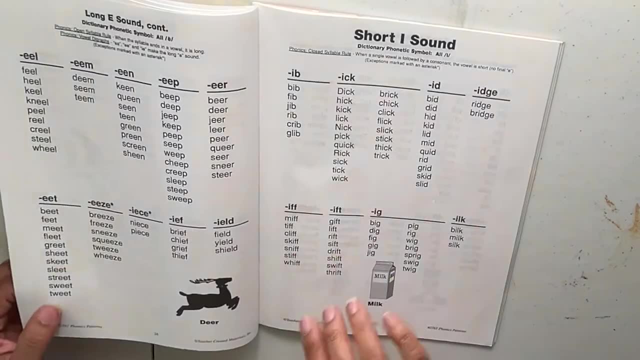 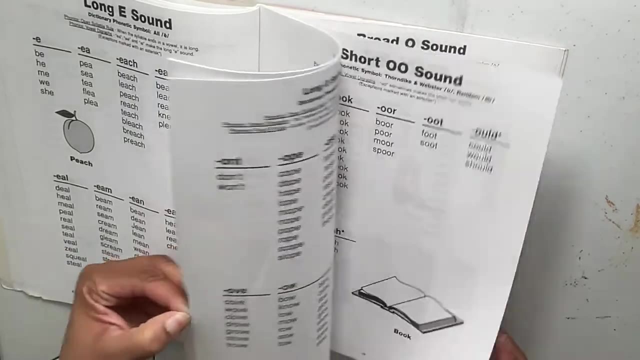 your kid or get them used to the at family. um, you know everything in here, eek e east, i mean it's a bunch of you know different word, families and you can actually break them down at the top. it has you know words with the long o sound or the short a or. you know whatever it may be. 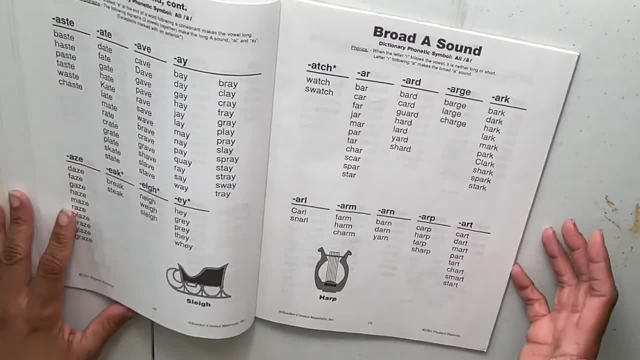 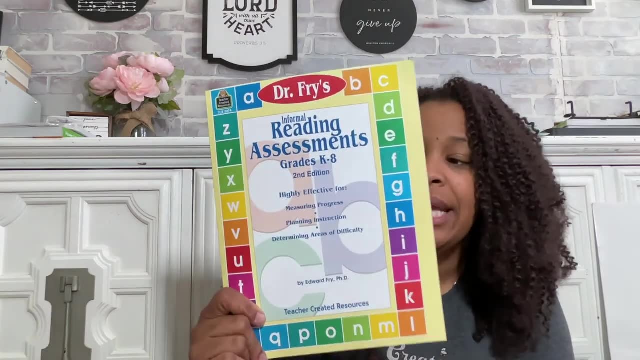 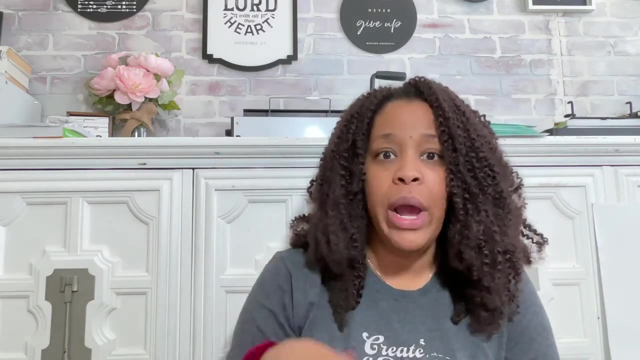 long a short a, and so we're using this for phonics. and then this is for our reading. we're using uh reading assessment, grades k through eight, and this is really cool because, again, this is kind of like this is an assessment book, so at least i know where um my kids are as far. 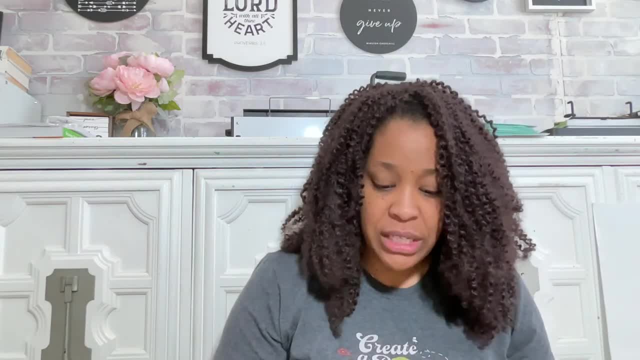 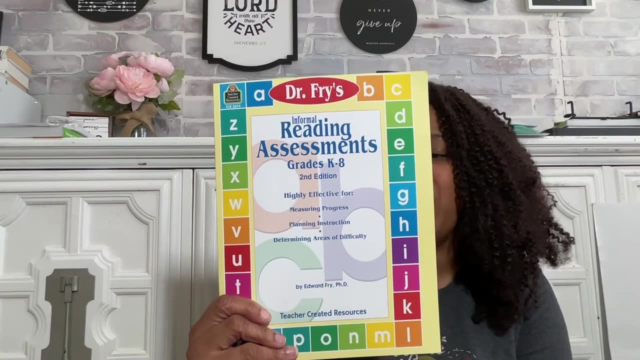 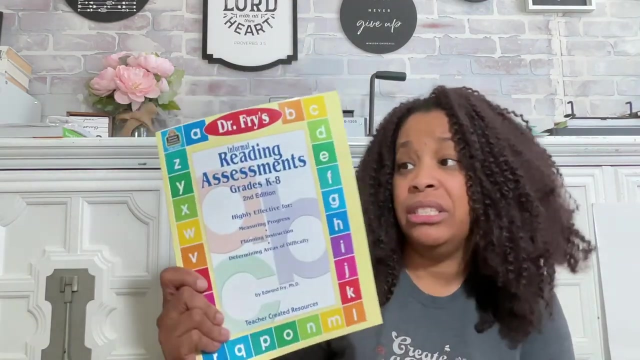 as they're reading what things we need to work on. so this book actually includes assessments for phonics, spelling, oral reading, phonemes, segmentation, letter and word recognition, onset and rhymes, comprehensions, homophones, vocabulary, hearing and vision. so this is a really cool book. so it's just basically it's an assessment book. 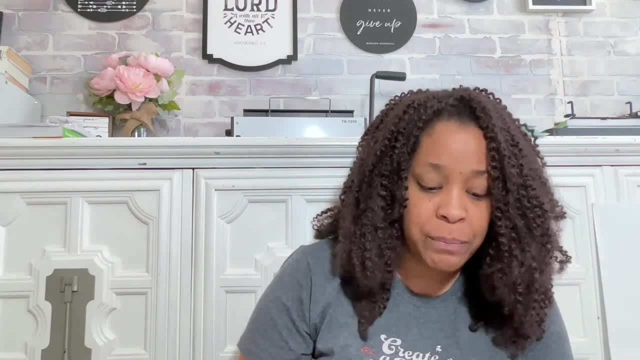 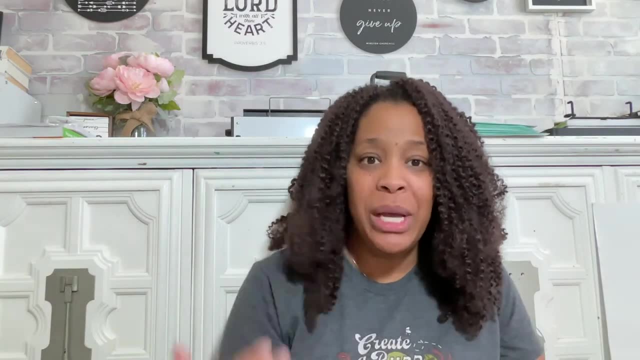 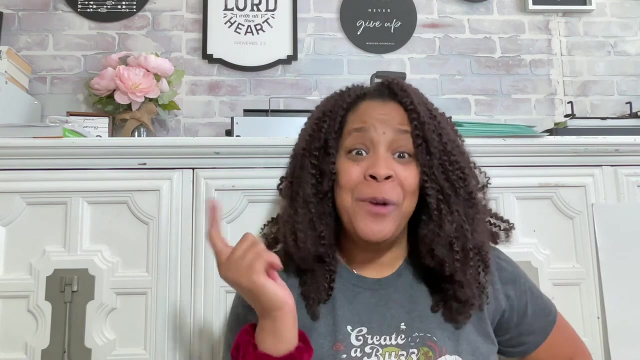 that way, um, we know where we want to start. yeah, so this is how we're kind of testing and making sure we're on par. so that is what i'm using to build our curriculum, what we're using as our base, as our foundation, so i know what needs to be taught. um, when does it need to be taught, kind? 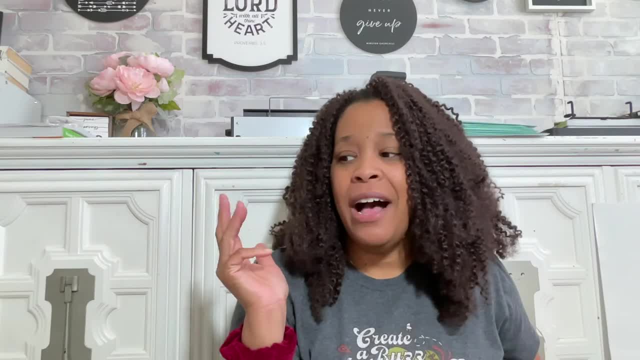 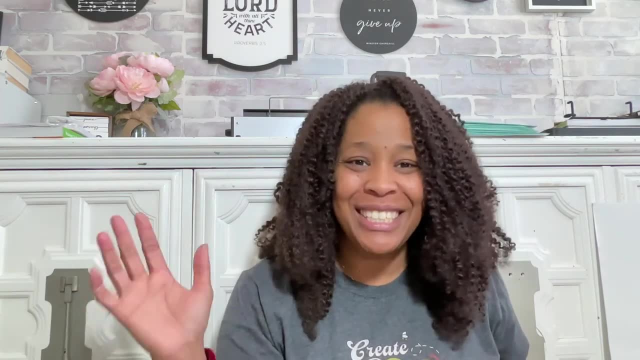 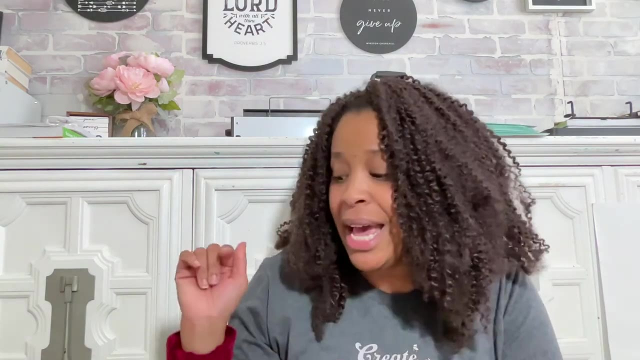 of help me in the order of how to teach it and making sure that they have actually understood and learned said topic for language arts. so that's it, guys. um, i will link everything down below. everything that i can will be linked down below in the description if you have any questions about anything i've said in. 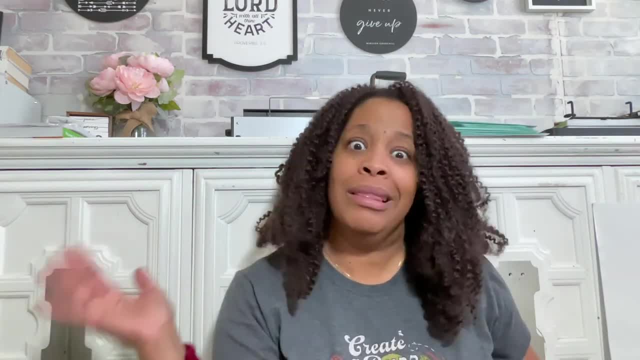 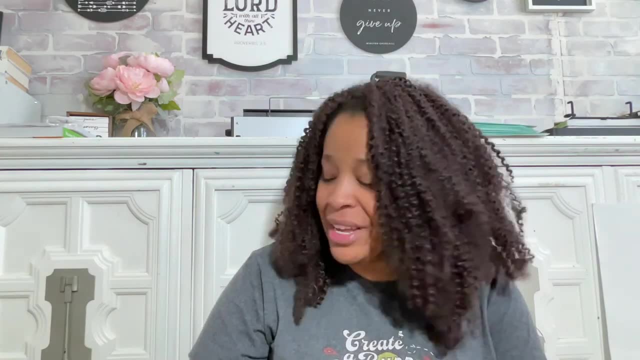 this video, anything i've shown in this video or just something that you think will relate to this video? um, just drop that down below and i can answer that for you again. um, it's a journey and we're figuring out how to teach it and i'm going to be doing that in the next couple of weeks. 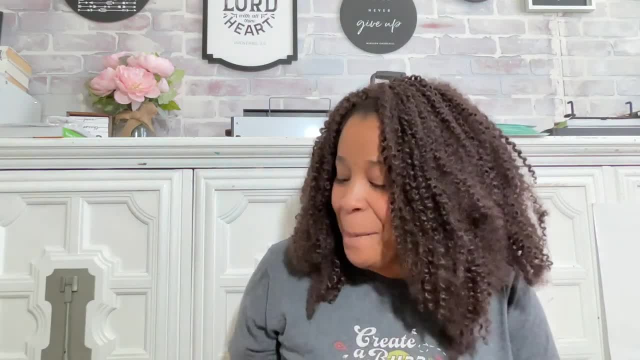 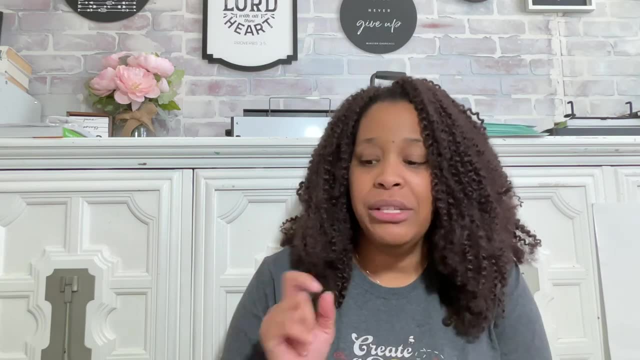 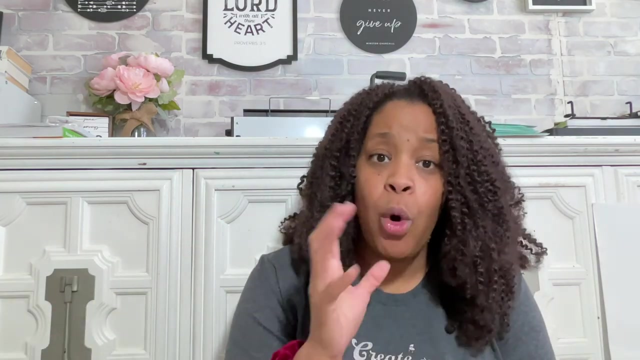 so stay tuned. i will be posting up um pretty soon just what we are using for our kindergarten curriculum, as well as our third grade curriculum, and that will show you more detail on that specific things for that grade level. this was just an overview of the resources that we are using to